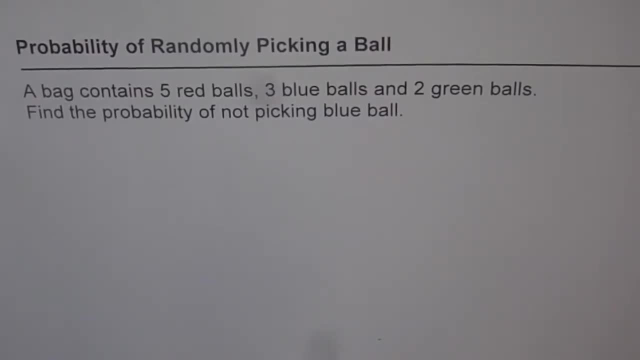 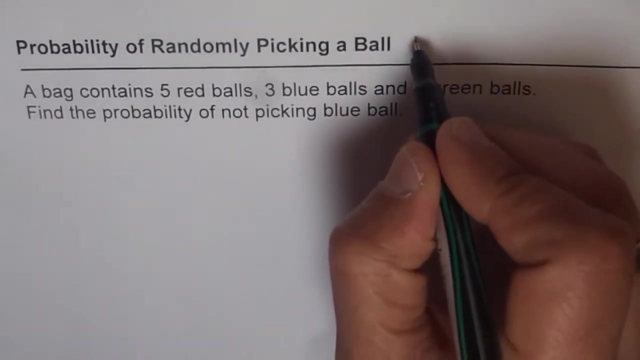 Probability of randomly picking a ball. The question here is: a bag contains five red balls, three blue balls and two green balls. Find the probability of not picking blue ball. So it is basically not picking. It's not just picking a blue ball, It is in fact not picking a blue ball. 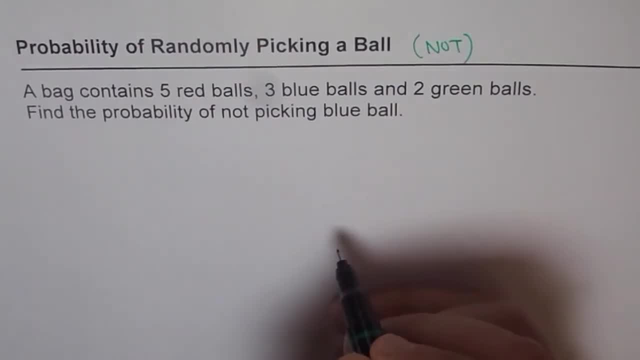 right. So that is the question for us. How do we do these kinds of questions? So let's start with making type of diagram for us. How many red balls do we have? We have five red balls, right. So let's randomly put five red balls right, So we got five red balls. How many blue balls? Three, right, So. 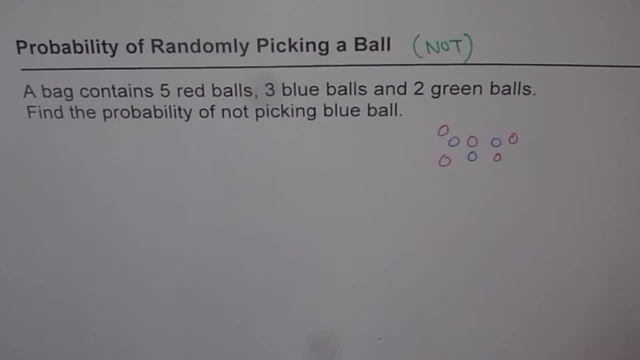 let's put three in our bag and there are two green balls. So we have two green balls here. So in all, how many do we have here? In all, we have five plus three plus two, and that gives us ten, So that. 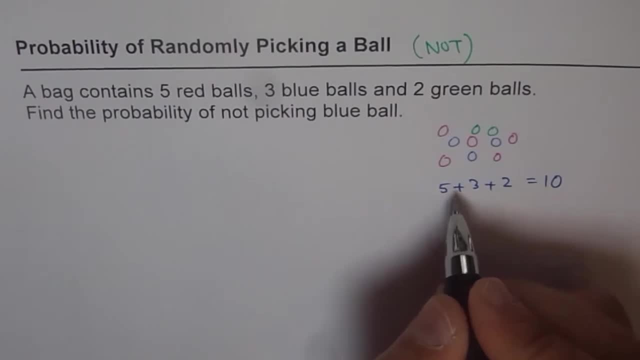 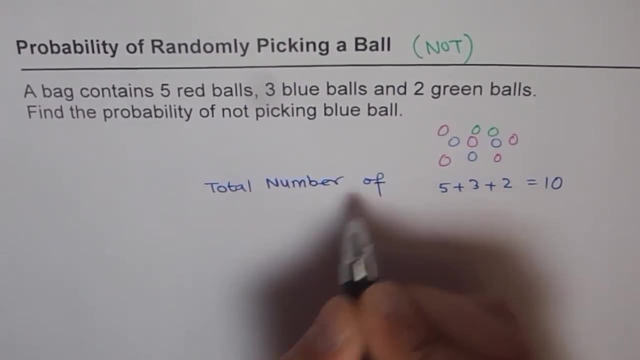 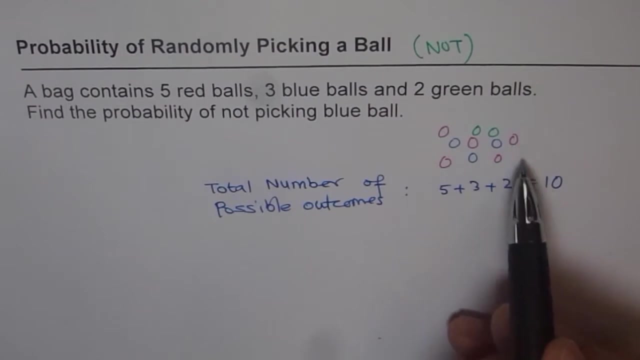 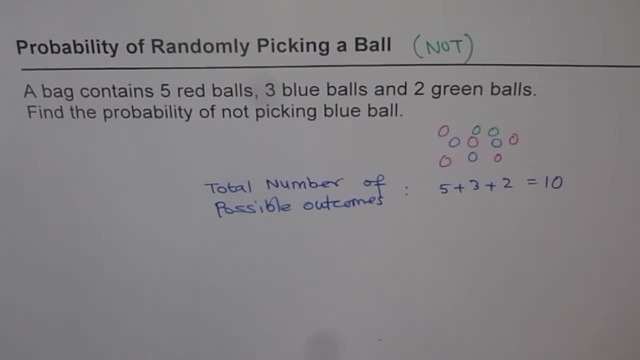 outcomes right, So these are all possible outcomes right, So these are all possible outcomes. right, So, these are all possible. picking blue ball: So how will you do that? So we can have two approaches here. So that is, we can. 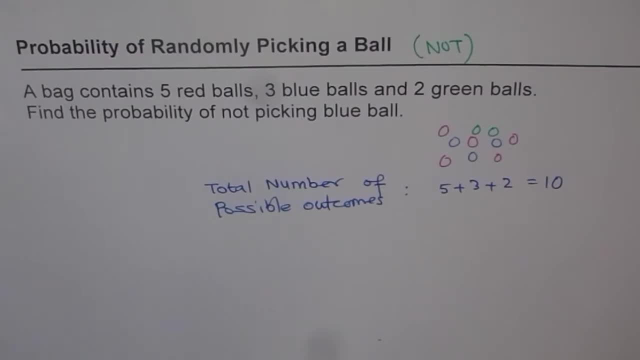 find probability of picking blue ball and then from there get the probability of not picking blue ball. So that is one of our approach. So that seems to be good, Let's do that. So first approach we'll do is probability of picking blue ball. So we say probability of picking blue ball. 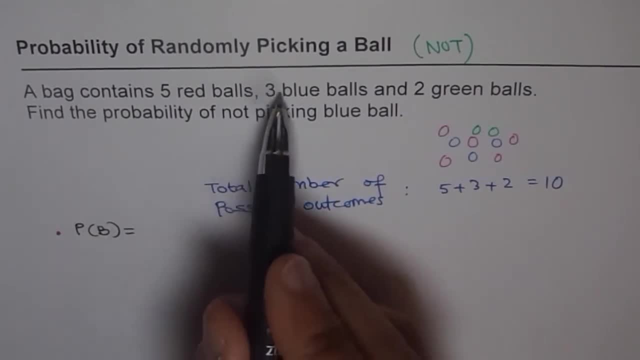 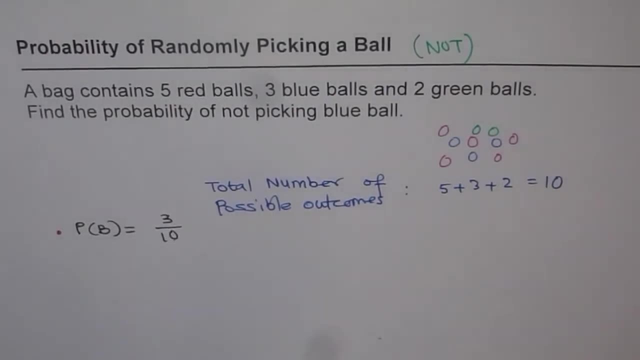 is what. So it is, how many number of blue balls are there? One, two, three right, And what are total number of balls? Ten. So three over ten is the probability of picking a blue ball, But what we want is of not picking. So probability of not blue is what It should be: one minus three over. 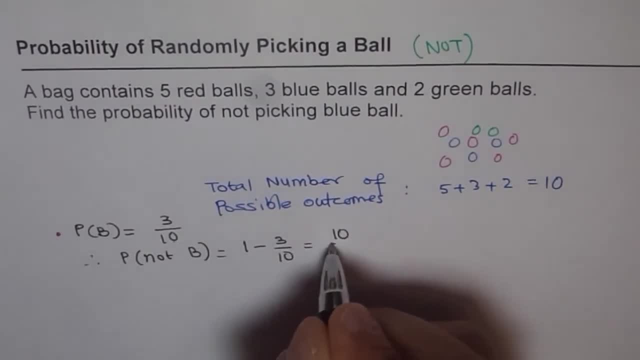 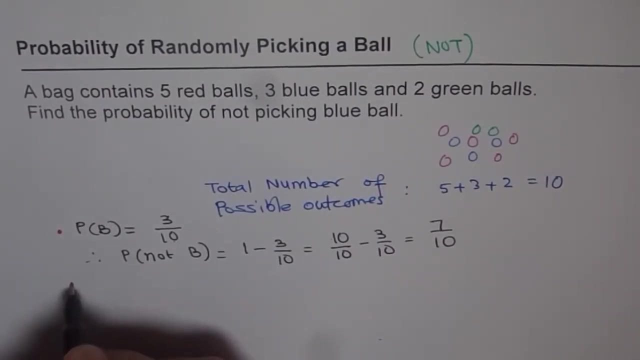 ten, correct: One minus three over ten. That gives us ten over ten Minus three over ten and that is seven over ten. So that is our answer for the given question. This is one way of doing it. Let me show you another way of doing the same thing: right? Alternate. 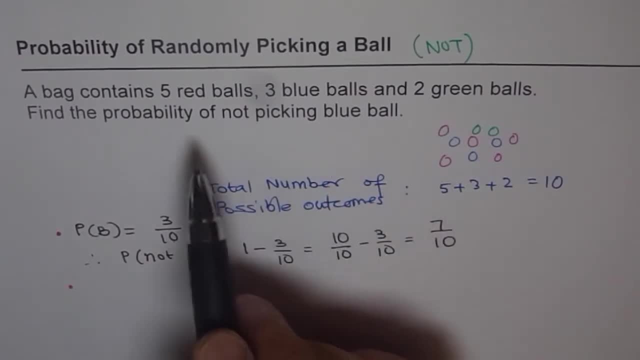 way is. in this particular case, we have three kinds of balls, That is, we have red, blue and green. So if you don't pick blue, what will you pick? You will pick either red or green, Do you see that? So what we can do is we can pick either red or green. So what we can do is we can pick either. 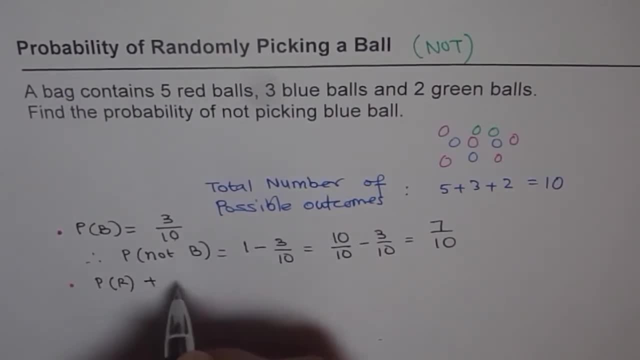 red or green. So what we can do is we can pick either red or green. So what we can do is we can find probability of picking red plus probability of picking green, add them up right And get the answer. So let's do that way. also. Probability of picking red is five out of ten, right, And that of 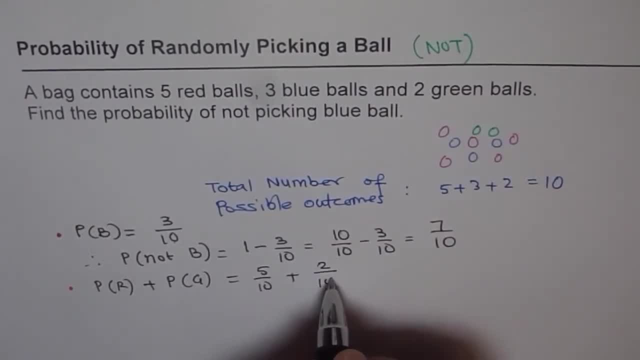 green is there are two green balls, so two out of ten. So which gives us seven over ten. So we get exactly the same answer. Do you see that? So when a question is like this, you could do it either way. You get the same answer. Remember, probability of picking one of these is what Sum of all the? 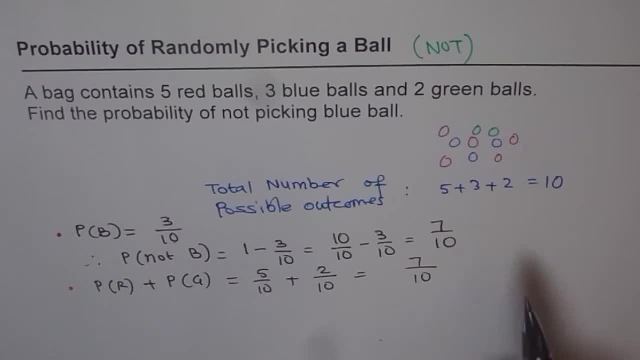 three, which will be one hundred percent right. One of these, of course, You are picking the balls, which is one of these. Now, picking only red will give you number of red divided by total. as you have seen here, Picking green will be two out of ten and blue is three out of ten. When you add 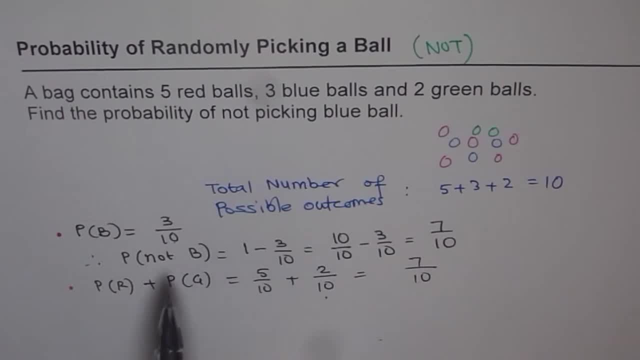 all of these together you get the answer. So we know that we can find the solution of these questions. let me repeat here, in two different ways. To find the probability of not picking means one minus picking Right, Because total sum is always one. So that is one approach which is a.